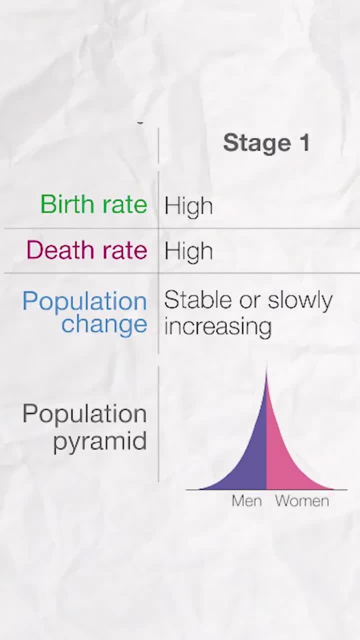 remember the four stages to this theory. In stage one, both birth rate and death rate are high, leading to little population growth. In stage two, the death rate starts to fall due to improved access to healthcare, sanitation and improved food supply. And since birth rate still remains, 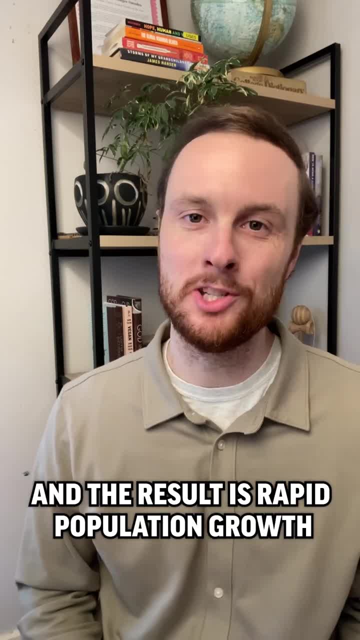 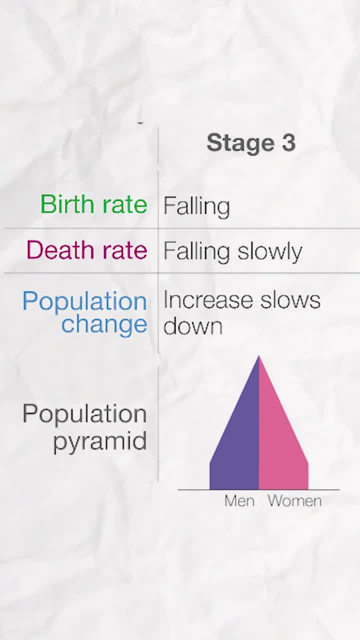 high. this means there are a lot more people being born than dying, and the result is rapid population growth. In stage three, the birth rate begins to fall due to increased educational opportunities for women, decreased infant mortality and increased access to contraception and family planning resources. This means that the population is still growing, but that rate. 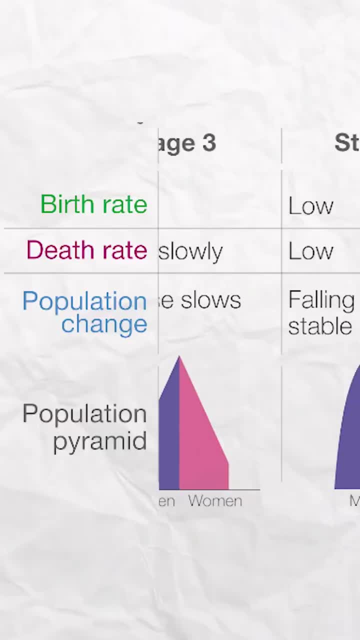 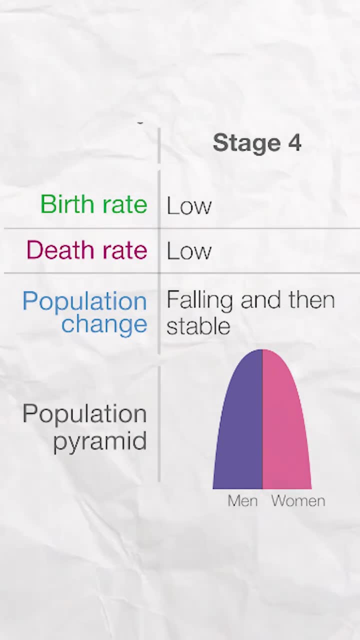 of growth is slowing down and the population is headed towards a stable size In stage four. countries have become so highly developed and affluent that birth rate drops even further and population growth goes to zero or even negative. If you want to learn more about the theory of demographic transition. check out my full video on YouTube. 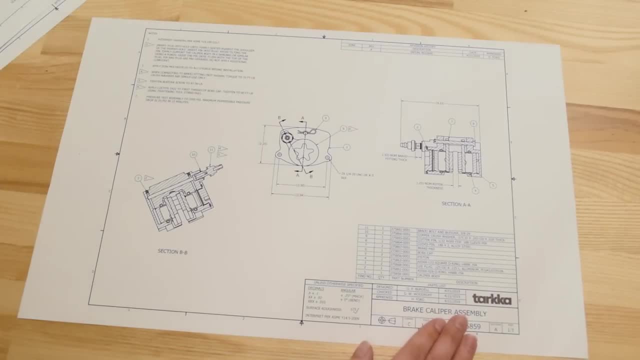 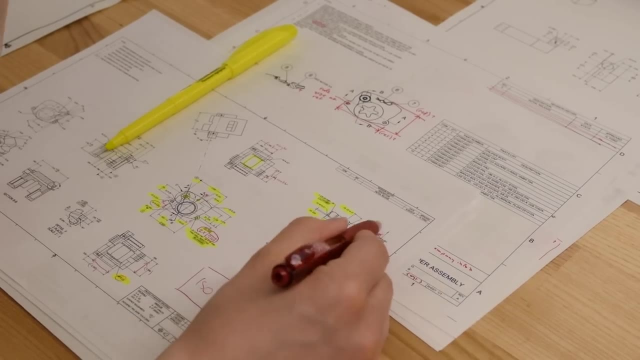 Engineering drawings are the most important deliverables that a design engineer produces. They provide all the instructions needed to make parts exactly as you intended. but bad drawings will make you look like a bad engineer and parts made from them are sure to have problems. In addition, many machine shops refuse to quote jobs that have bad drawings. 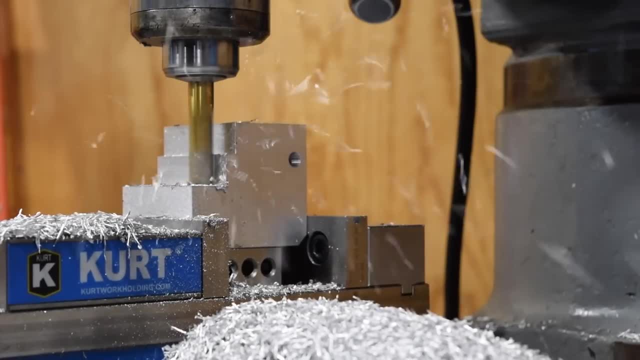 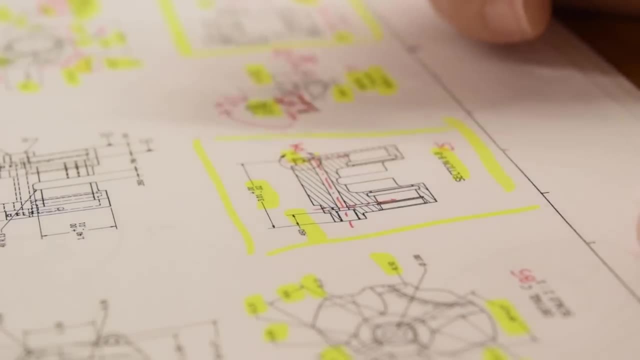 because nothing is more disruptive to them than having to call the engineer for missing dimensions or clarification. In this video, we're going to give you some tips for making clear, complete drawings, so you don't embarrass yourself. We tried to make this video as painless as 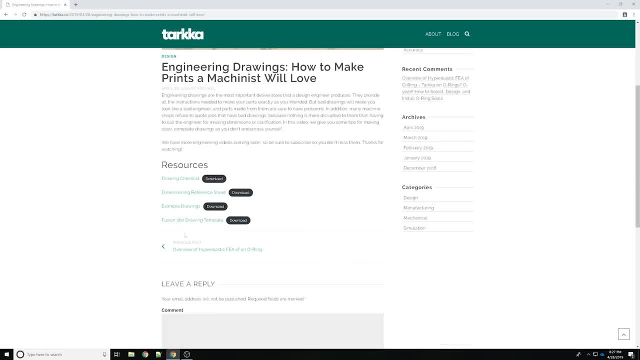 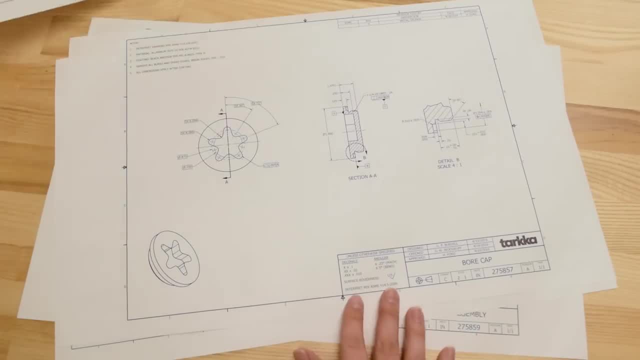 possible, so we've provided lots of extra resources on our website that cover the more tedious details. Our checklist will help ensure your drawings are complete, and this reference sheet shows some different ways to dimension common features. We've also provided a fully dimensioned drawing package with both detail and assembly prints to serve as an example. 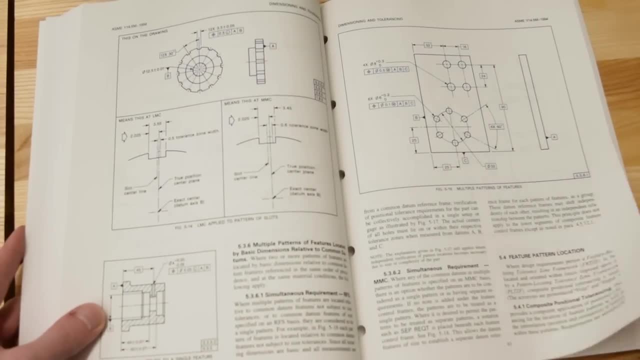 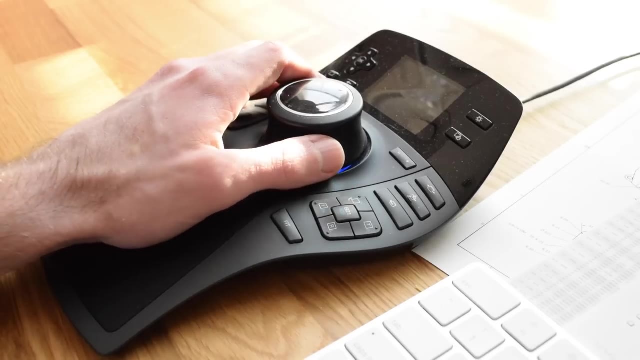 And if you really need to dive into the details, we've provided references to the relevant ASME drafting standards throughout the video. These days, the vast majority of 2D drawings are made in the computer from a 3D parametric CAD model. In this video, we're going to be using Autodesk. 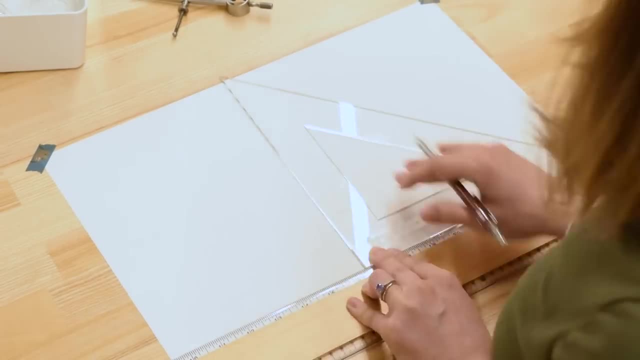 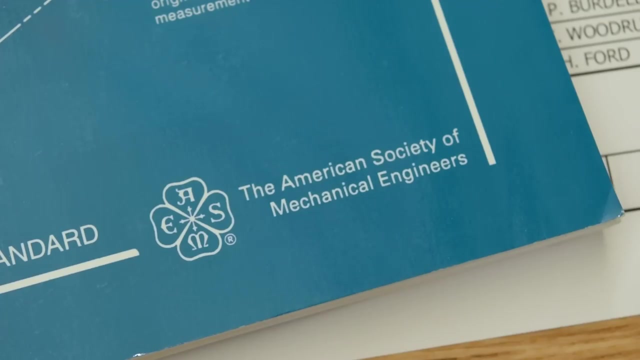 information we're giving you applies to any software package or even hand drafting. If you're new to CAD, Fusion 360 is free for hobbyists and startups and is a great option. We're going to be working to the drafting standards of the American Society for Mechanical.